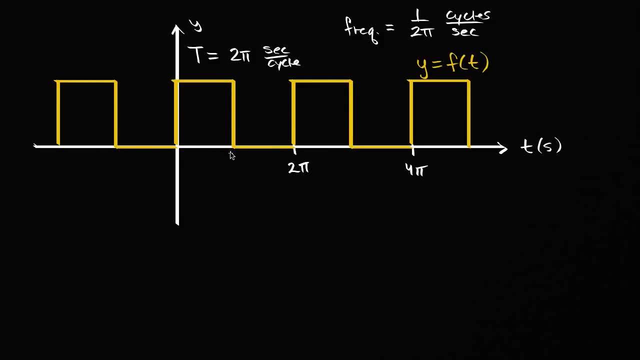 is, can we take a periodic function like this and represent it as an infinite sum of sines and cosines, of different periods or different frequencies? So to write that out a little bit more clearly, can we take our f of t? So can we take our f of t and write it. 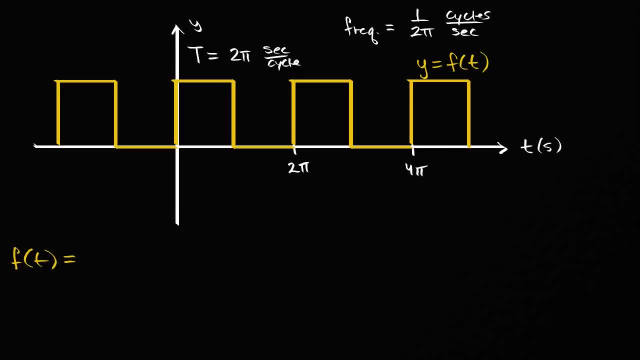 as the sum of sines and cosines. So can we write it. so it's going to be some, let's say, baseline constant That'll shift it up or down And, as we'll see, that's going to be based on the average value of the function over one period. 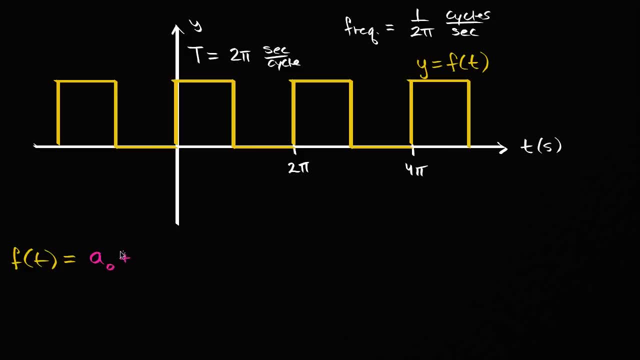 So a sub zero. And then let's start adding some periodic functions here, And so let's take a sub one times cosine of t. Now, why am I starting with cosine of t? And I could also add a sine of t. So plus b, sub one. 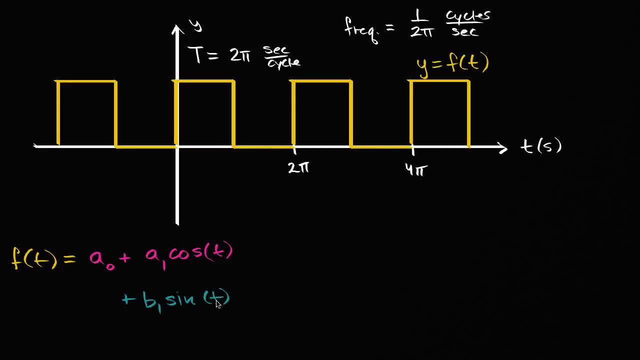 plus b sub one of sine of t. Why am I starting with cosine of t and sine of t? Well, if our original function has a period of two pi- and I just set up this one, so it does have a period of two pi. 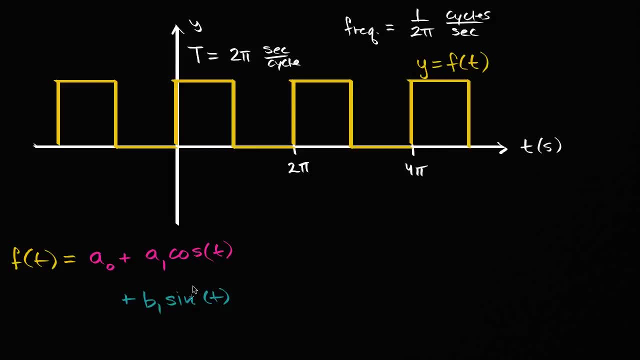 well, it would make sense that it would involve some functions that have periods of two pi, And these weights will tell us how much they involve it. If a one is much larger than b one, well it says, okay, this has a lot more of cosine of t in it. 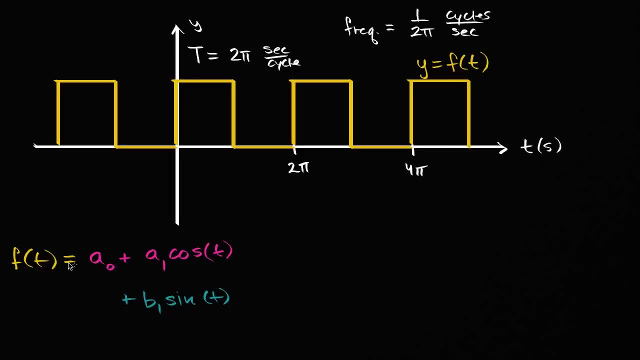 than it has of sine, of t in it, And that by itself isn't going to describe this function, because we know what this would look like. This would look like a very clean sinusoid, not like a square wave, And so what we're going to do is we're going to add: 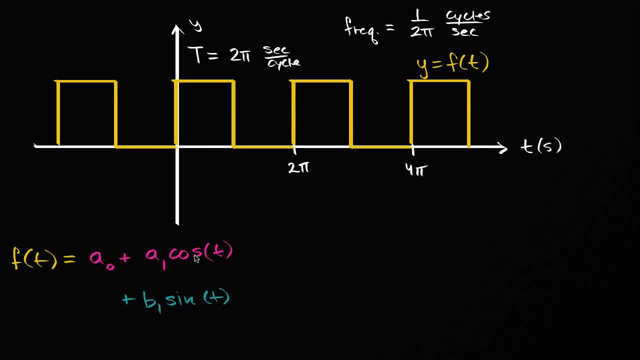 we're going to add sinusoids of frequencies that are multiples of these frequencies. So let's add, let's add a sub two, so another weighting coefficient times cosine of two. t, This has a frequency of one over two pi, This has twice the frequency. 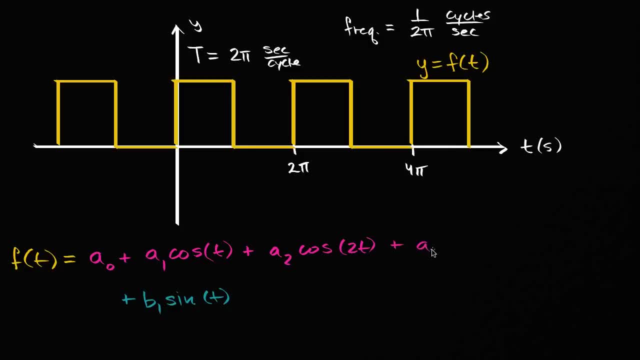 This has a frequency of one over pi, And then a sub three times cosine of three t, And I'm going to keep going on and on and on forever, And I'm going to do the same thing with the sines. So, plus b, two, sine of two t. 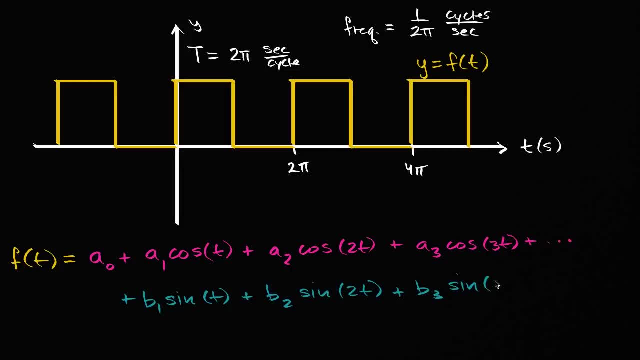 Plus b, three sine of three t, And you might be saying, well, okay, this seems like a fun little mathematical exercise, but why do folks even do this? Well, this was first explored and they're named series like this infinite series where you represent something. 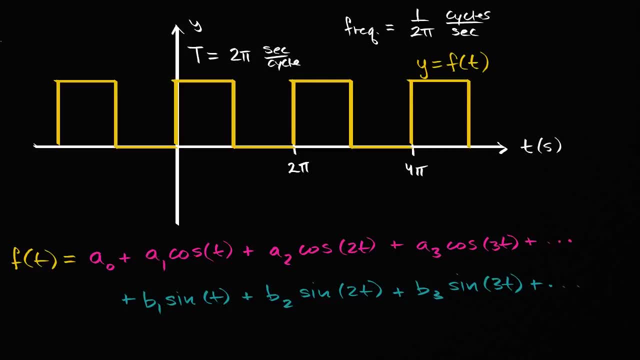 by essentially weighted sines and cosines. This was explored originally by Fourier and they're called Fourier series And they were interesting to him in the study of differential equations Because a lot of differential equations are easy to solve when you involve sines and cosines. 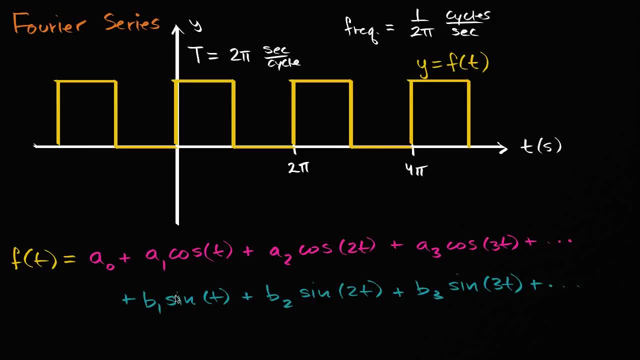 are easy to solve when you involve sines and cosines, but not as obvious to solve when you have more general functions, like maybe a square wave here. But if you could represent that square wave as sums of sines and cosines, then all of a sudden you might be able to find 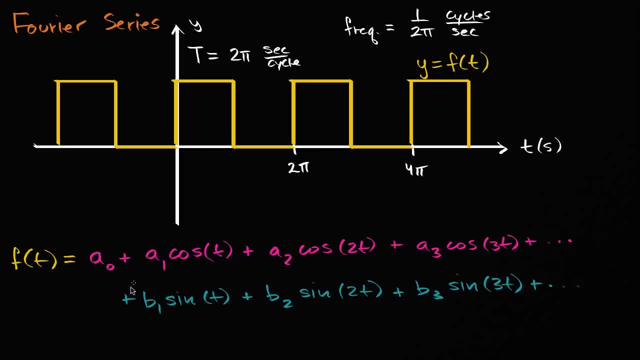 more general solutions to your differential equations. Another really interesting thing about this- and this is really the foundation of signal processing, it's very used, it's heavily used in electrical engineering- is you can view these coefficients as they are. they're weights on these cosines and sines. 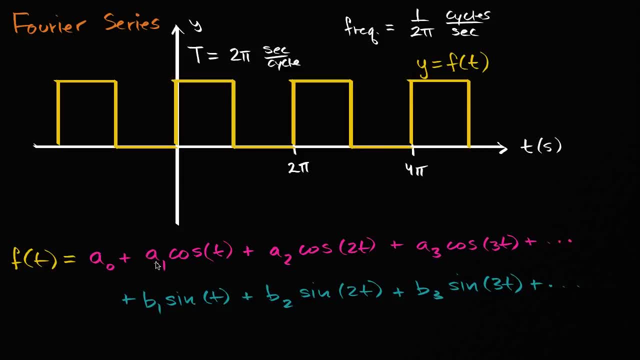 but another way to think about it is they tell you how much of different frequencies that this function contains. So, for example, if a1 is much bigger than a2, then that tells you that that function contains a lot more of the one over two pi hertz frequency. 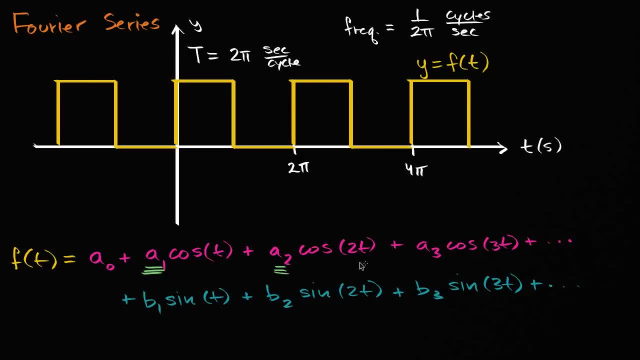 than the one over pi frequency, Or maybe a2, or maybe a3 is bigger than a1 or a2.. And so you can start to say: hey, this helps us think of a function not just in terms of the time domain, which f of t does. 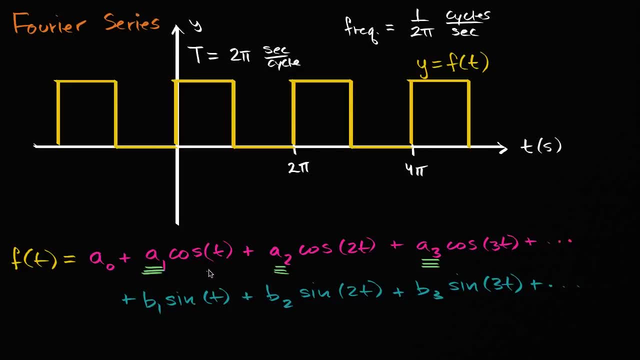 but it can start bringing us to saying: well, how much do we have of each frequency? And, as we'll see, with Fourier series and eventually Fourier transforms, that's going to get us into the frequency domain where we can start doing some signal processing. 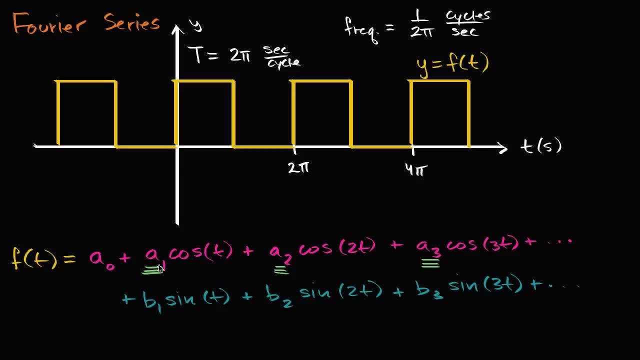 So we're going to explore all of that in future videos In order to understand how we can actually find these coefficients. we're going to review a little bit of our trigonometry, especially integrating trig functions, and then we're going to solve for these. 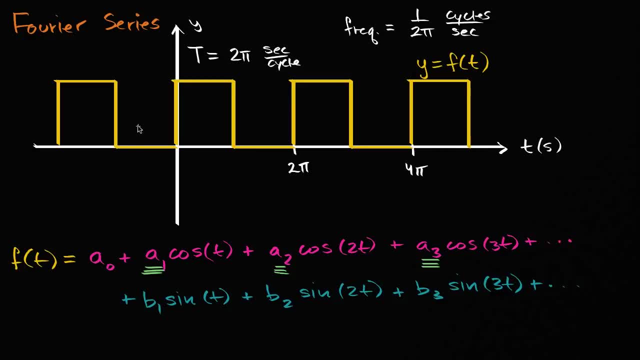 and we're going to see how good we can approximate our function f.